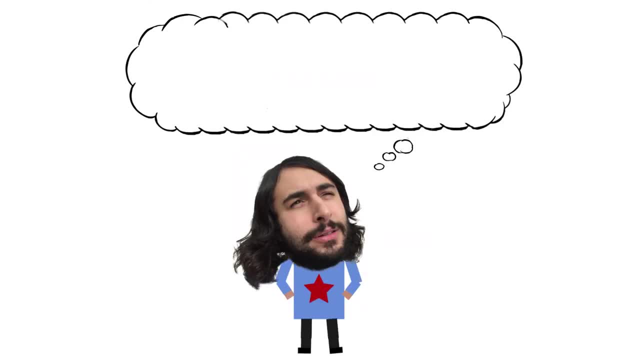 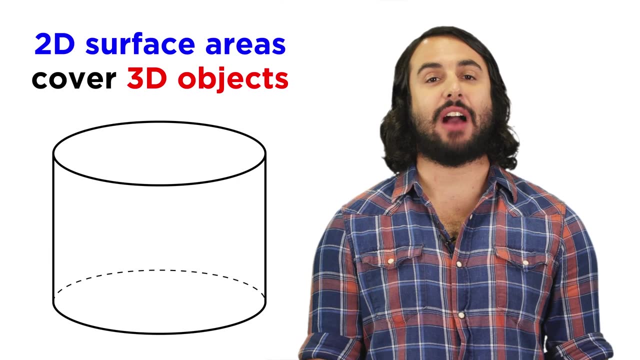 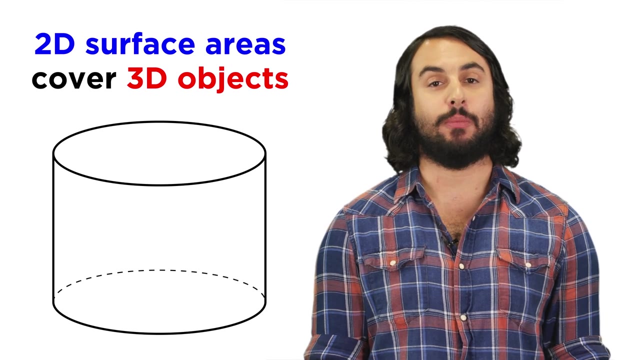 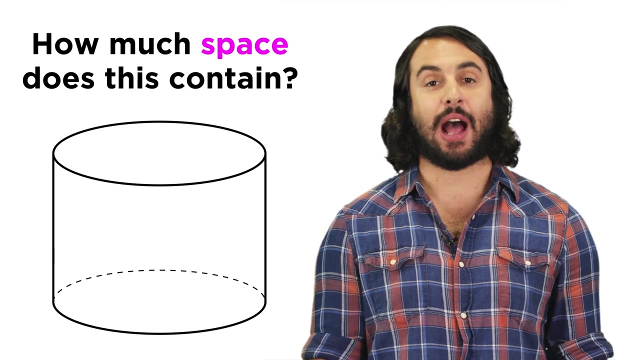 Professor Dave, again let's talk about volume. We just learned how to calculate the two-dimensional area covered by the surface of a three-dimensional object, but sometimes we want to do more than that. Sometimes we want to calculate the three-dimensional space that is contained within that object. 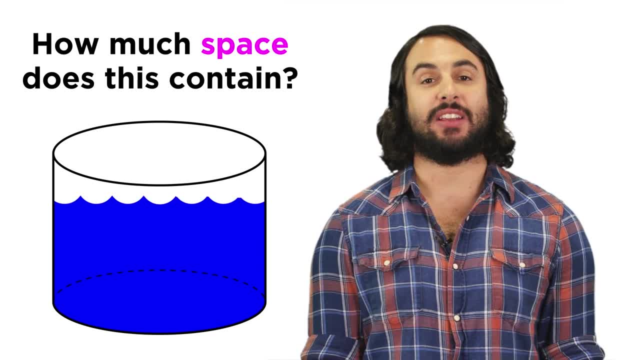 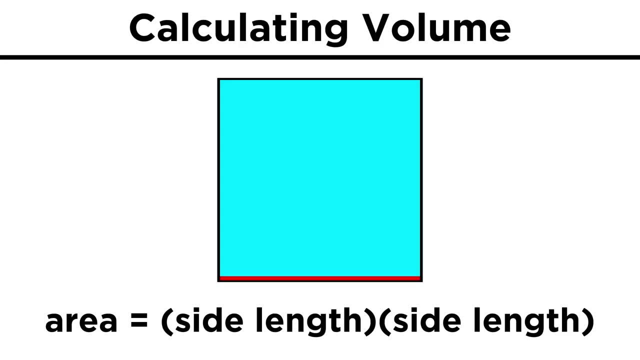 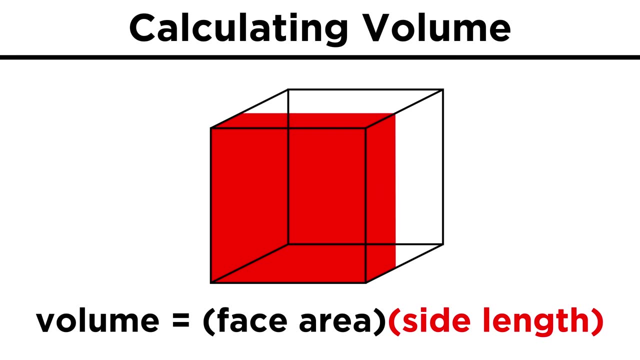 which we can think of as the amount of water we will need to fill up the object if it were perfectly hollow. Just the way the area of a square is found by running a side length across the shape. if we take that square surface and run it across a third dimension, we can get a cube. 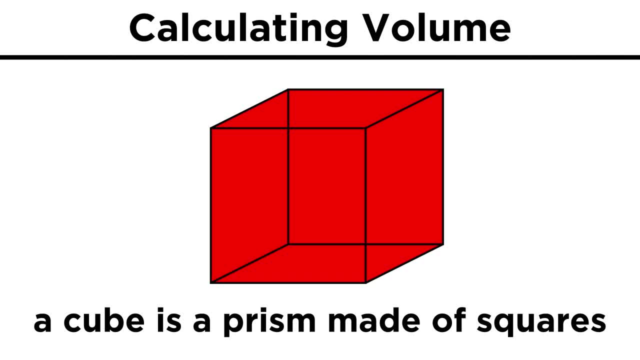 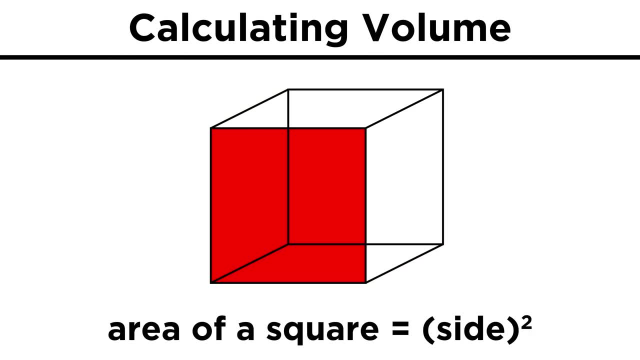 A cube is a prism with squares for all its faces. To find the volume of a cube, instead of just squaring the side length, we need to find the side length which gives us the area of one square face. we cube the side length to. 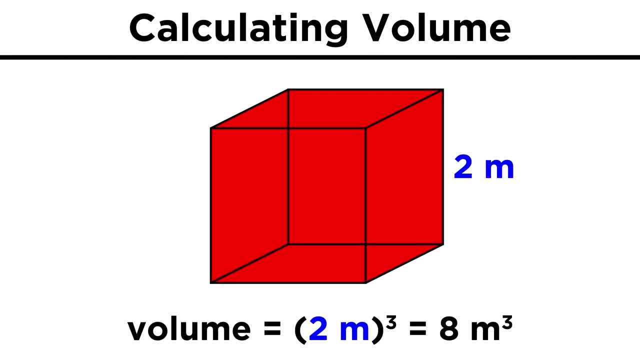 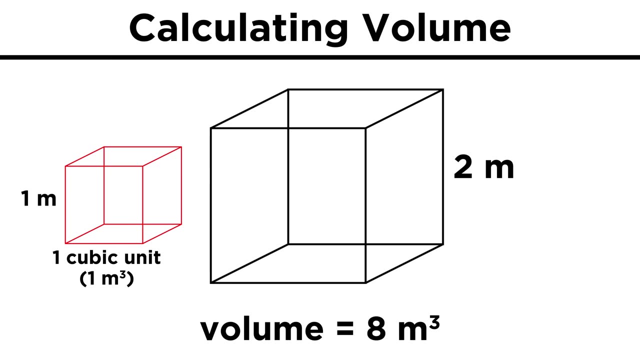 get the volume of the cube. With a side length of two meters, this cube has a volume of eight meters cubed or cubic meters. We can easily visualize this by saying that if we have some one by one by one cubes or cubic units, it will take eight of them to fill this larger cube. 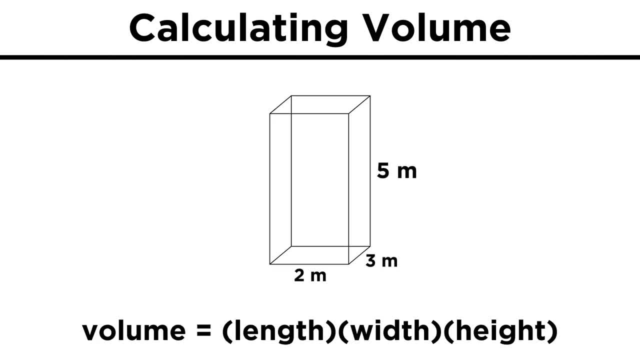 For a rectangular prism, it's just length times width times height. Two times three times five gives thirty cubic meters. What we are really doing is calculating the area of the base and multiplying by the height, as though running the base up through the height of the shape to span its volume. 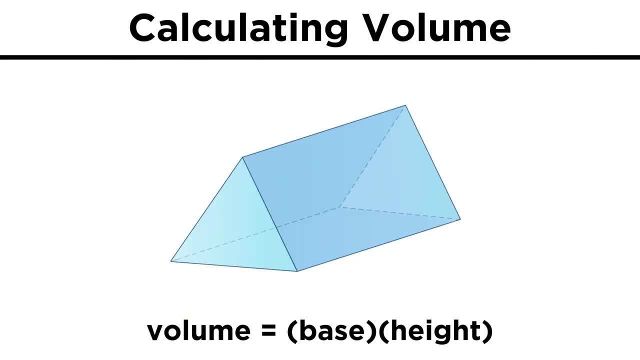 This works for any type of prism, Like a triangular prism. Here we have triangular bases, so we just get the area of one base and multiply by the height. If the triangle itself has a base and height of two and three meters and the prism has, 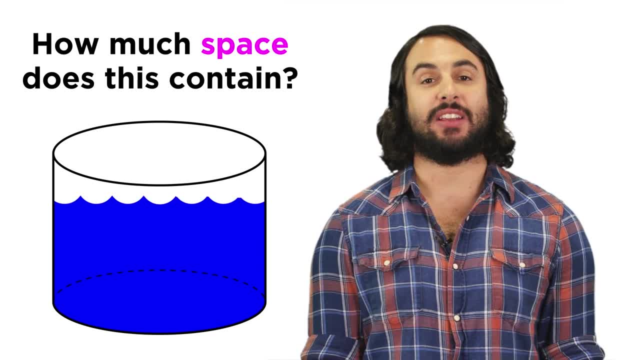 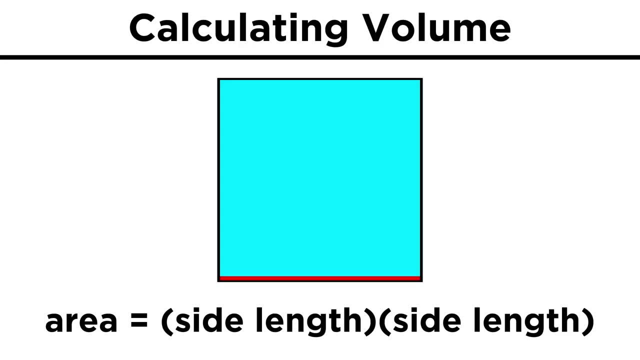 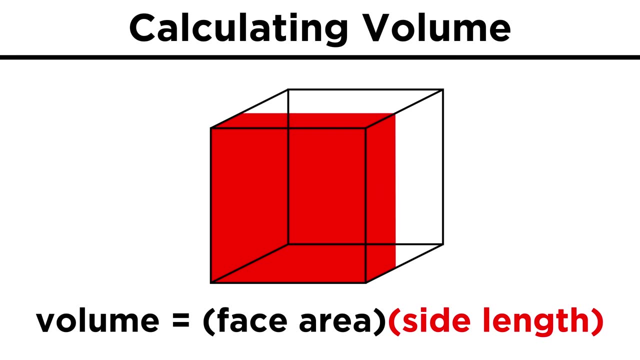 which we can think of as the amount of water we will need to fill up the object if it were perfectly hollow. Just the way the area of a square is found by running a side length across the shape. if we take that square surface and run it across a third dimension, we can get a cube. 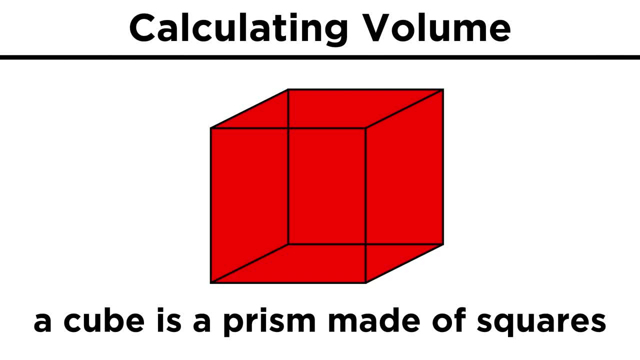 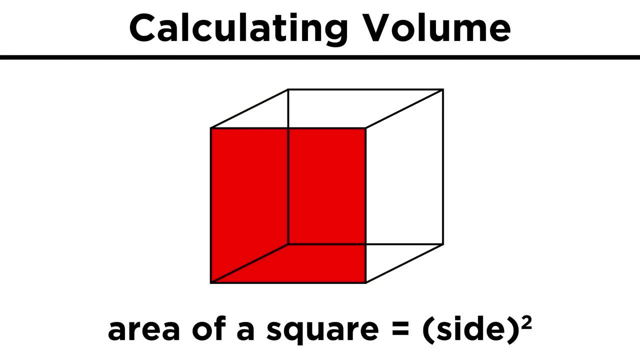 A cube is a prism with squares for all its faces. To find the volume of a cube, instead of just squaring the side length, we need to find the side length which gives us the area of one square face. we cube the side length. 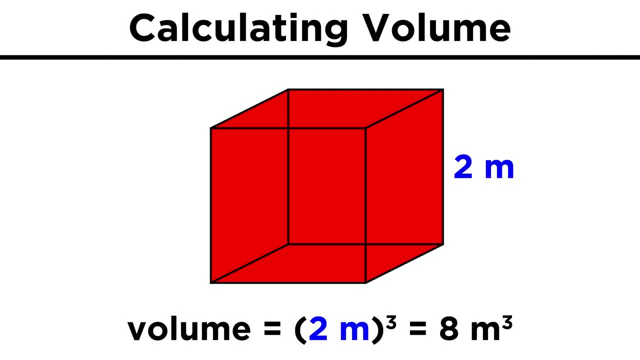 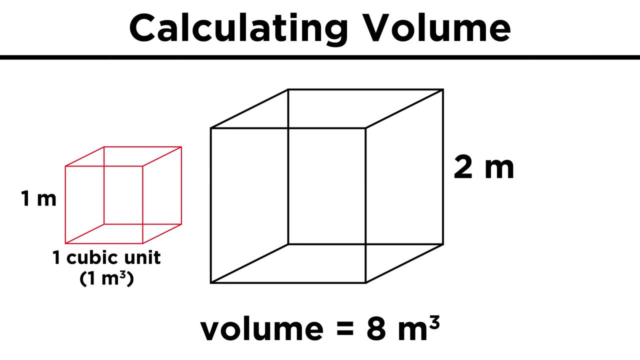 to get the volume of the cube. With a side length of two meters, this cube has a volume of eight meters cubed or cubic meters. We can easily visualize this by saying that if we have some one by one by one cubes or 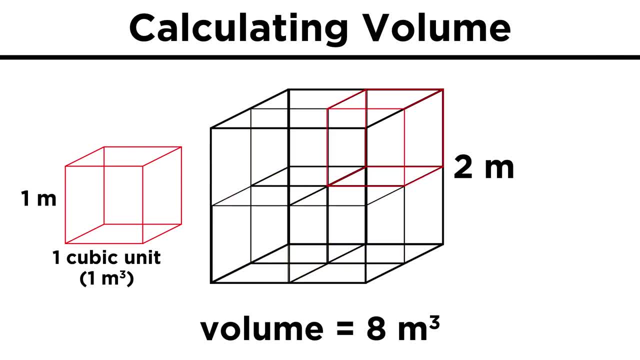 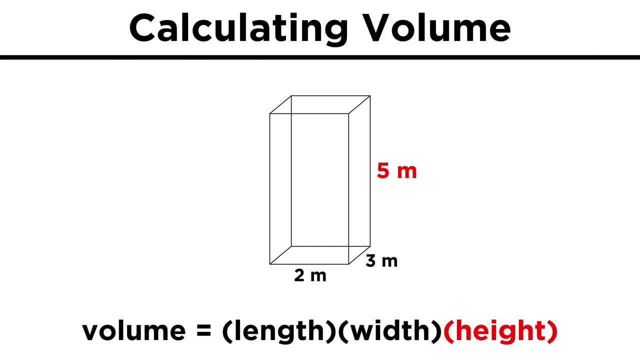 cubic units, it will take eight of them to fill this larger cube For a rectangular prism. it's just length times width times height. Two times three times five gives thirty cubic meters. What we are really doing is calculating the area of the base and multiplying by the height. 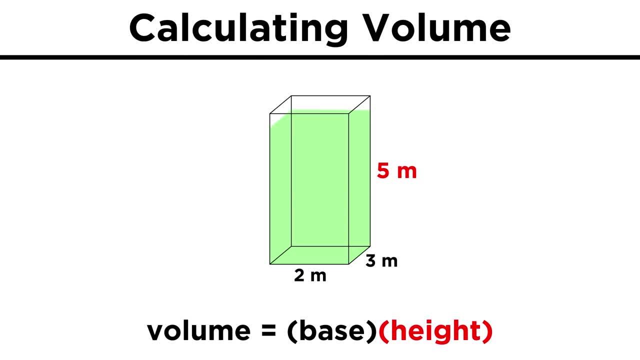 as though running the base up through the height of the shape to span its volume. This works for any type of prism, Like a triangular prism. Here we have triangular bases, so we just get the area of one base and multiply by the height. 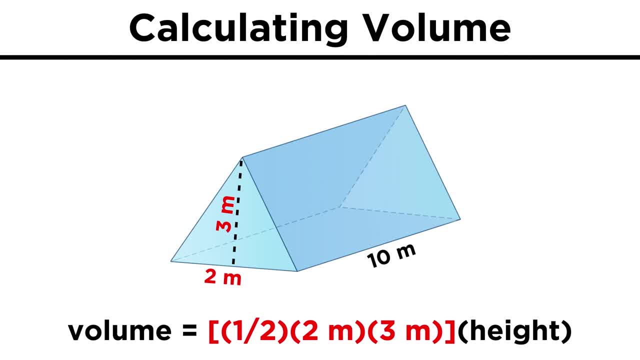 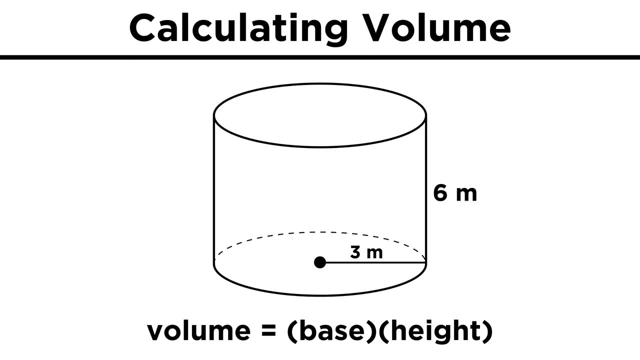 If the triangle itself has a base and height of two and three meters and the prism has a height of ten meters, we get one half, two times, three times ten or thirty cubic meters. This works for cylinders too. It's always just base times height. 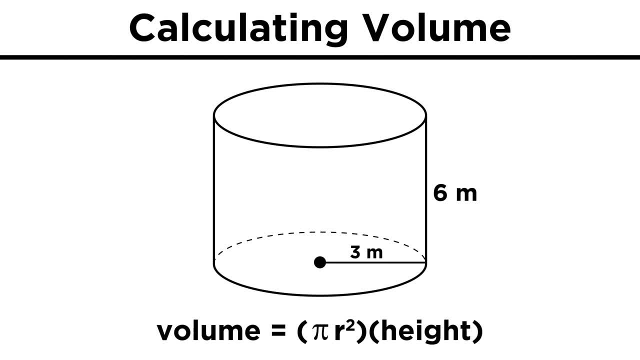 The base of a cylinder is a circle. so we find the area of this circle and then multiply by the height of the cylinder. If the height is six meters and the radius is three, we get pi R squared, or nine pi times six, or fifty four pi cubic meters. 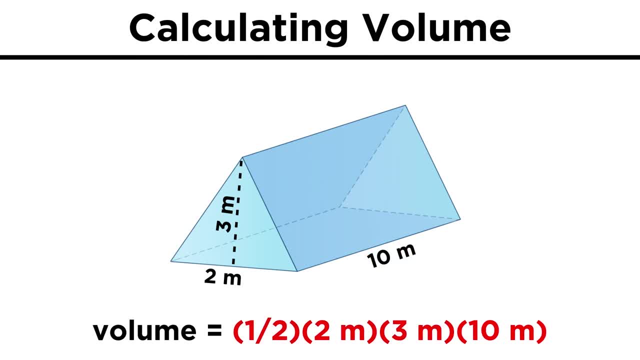 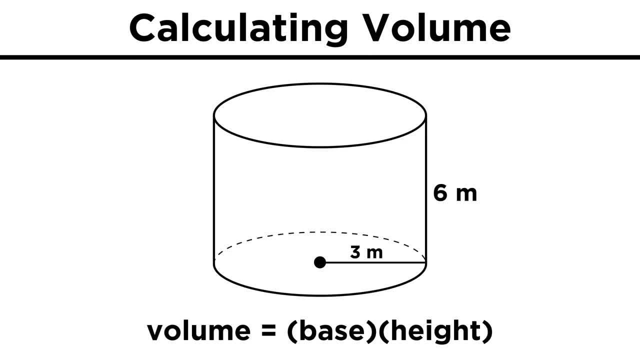 a height of ten meters, we get one half, two times, three times ten or thirty cubic meters. This works for cylinders too. It's always just base times height. The base of a cylinder is a circle, so we find the area of this circle and then multiply. 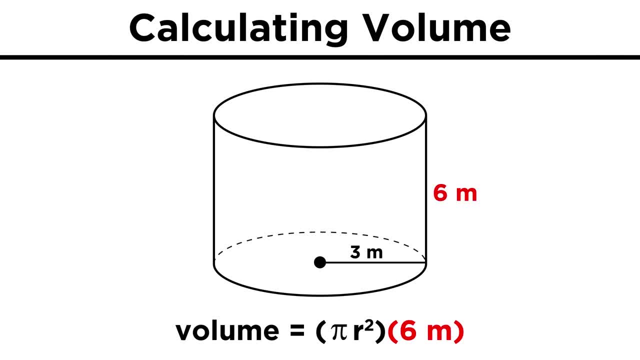 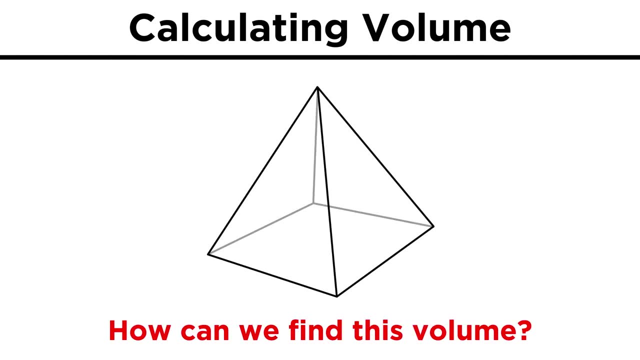 by the height of the cylinder. If the height is six meters and the radius is three, we get pi r squared, or nine pi times six or fifty-four pi cubic meters. Now let's move on to some trickier shapes. How do we calculate the volume of a cylinder? 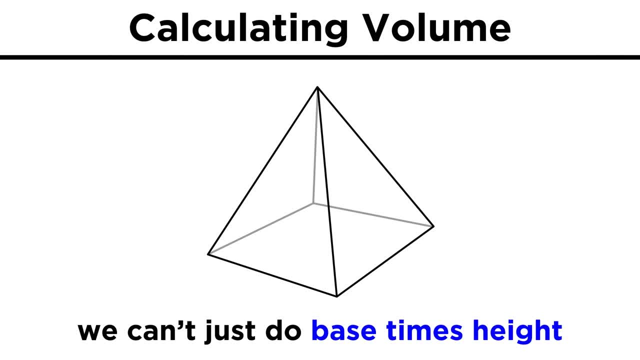 How do we calculate the volume of a pyramid? This will be different from a prism, because we can't just multiply the base times the height as the triangular faces slope inward. Instead, we will use the formula one: third base times height. So if we have a square pyramid which has a base with a length of three and the pyramid 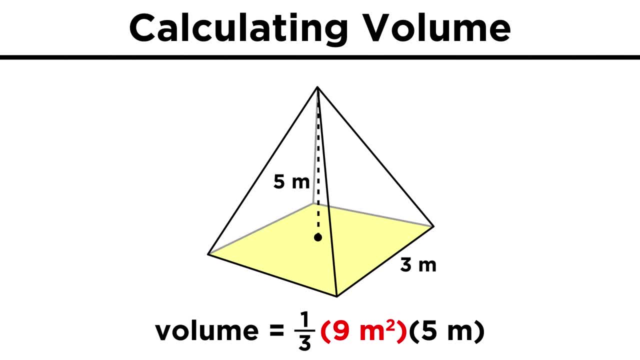 has a height of five, we get nine for the base Times. five is forty-five Times one third is fifteen cubic meters. What if we don't know the height of the pyramid, but only the height of the triangles? Luckily, we know the Pythagorean theorem, so we could imagine a triangle where one leg 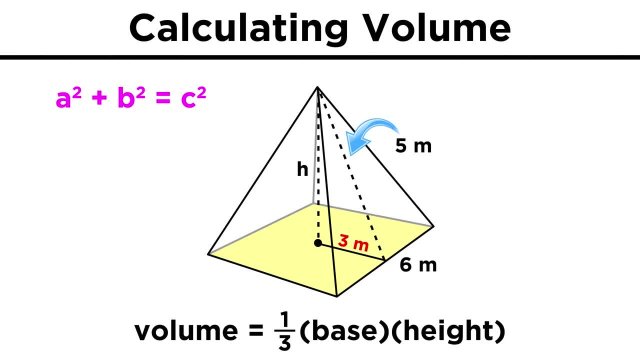 is the height of the pyramid, the other leg is half the length of the base and the hypotenuse is the height of a triangular face. We plug them into the equation and we can calculate the volume of the pyramid. So we can calculate the volume of the pyramid and we can calculate the height of the base. 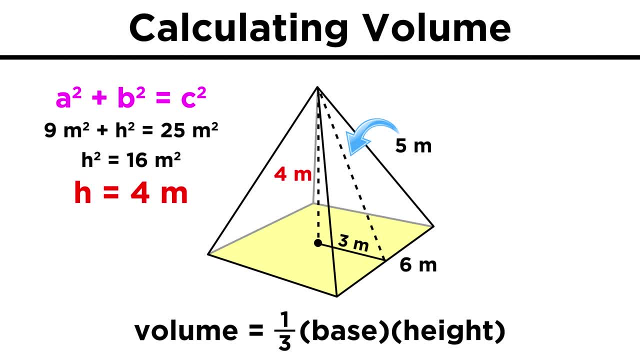 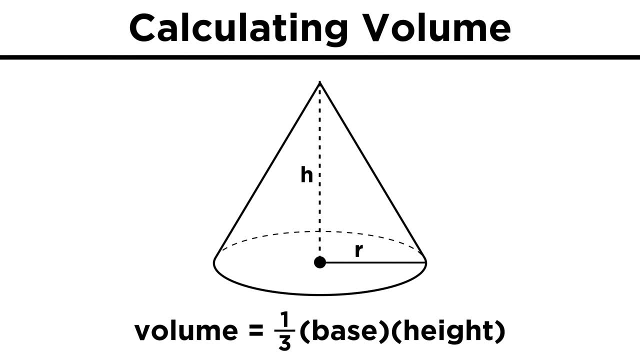 So we can calculate the volume of the pyramid. We can then solve for the height, So it's just one extra step. Cones work just like pyramids. Again, it will be one third base times height, except that here the area of the base is. 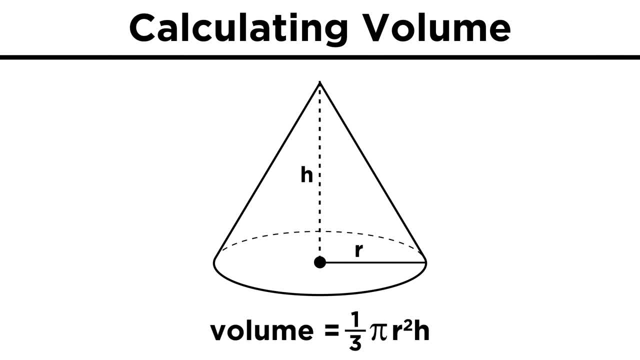 given by pi R squared. so we get one third pi R squared H. If we have two for R and nine for H, we get four pi times nine is thirty-six times a third is twelve cubic meters. Lastly, we need to be able to calculate the volume of a sphere. 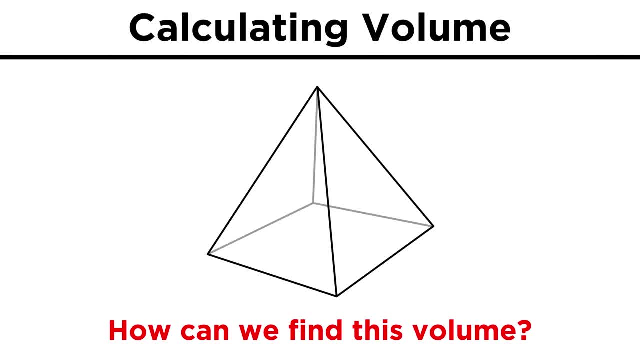 Now let's move on to some trickier shapes. The first one is the radius. The radius is three. The second one is the length of a pyramid. This will be different from a prism, because we can't just multiply the base times the 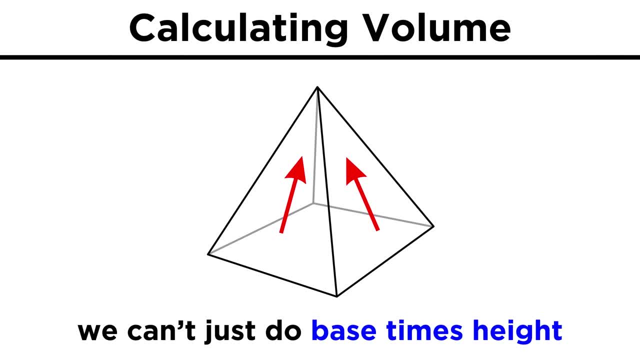 height as the triangular faces slope inward. Instead, we will use the formula one third base times height. So if we have a square pyramid which has a base with a length of three and the pyramid has a height of five, we get nine for the base times. five is forty five times one. 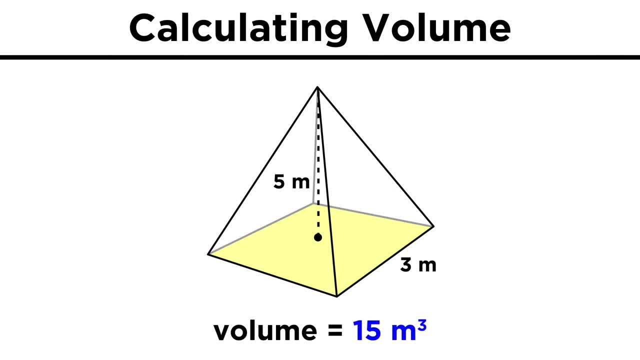 third is fifteen two, That's twenty cubic meters. What if we don't know the height of the pyramid, but only the height of the triangles? Luckily we know the Pythagorean theorem, so we could imagine a triangle where one leg is the height of the pyramid, the other leg is half the length of the base and the hypotenuse. 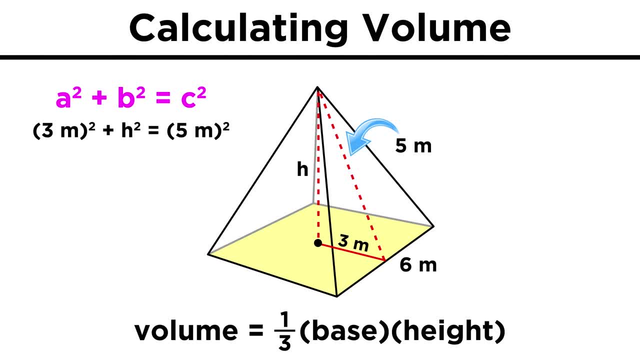 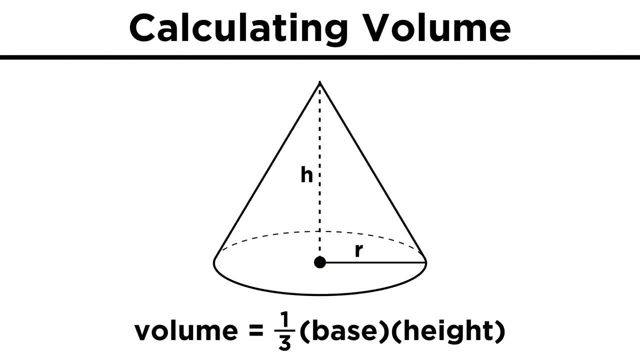 So it's just one extra step. Cones work just like pyramids. Again, it will be one third base times height, except that here the area of the base is given by pi R squared. so we get one third pi R squared H If we have two for R and nine. 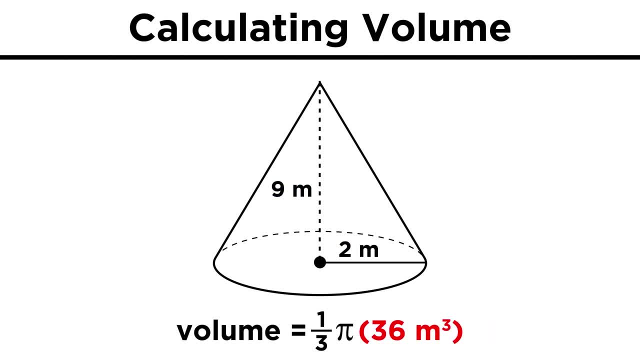 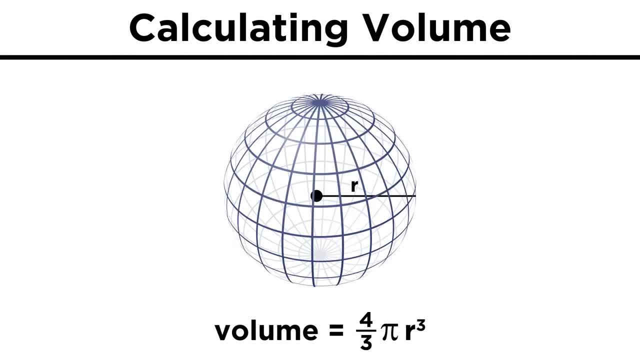 for H, we get four pi times nine is thirty. six times a third is twelve cubic meters. Lastly, we need to be able to calculate the volume of a sphere. The formula for this is four thirds pi R, cubed. So with a radius of three. we cube it to get twenty seven. divide by three to get nine. 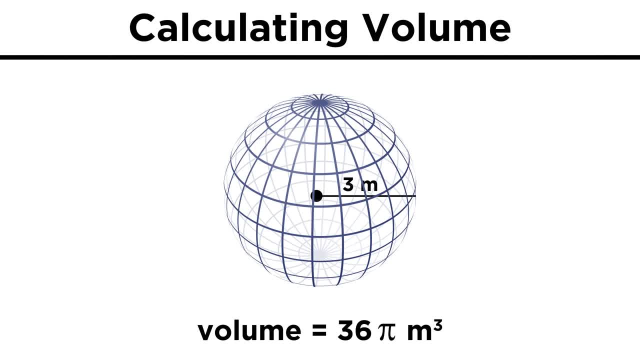 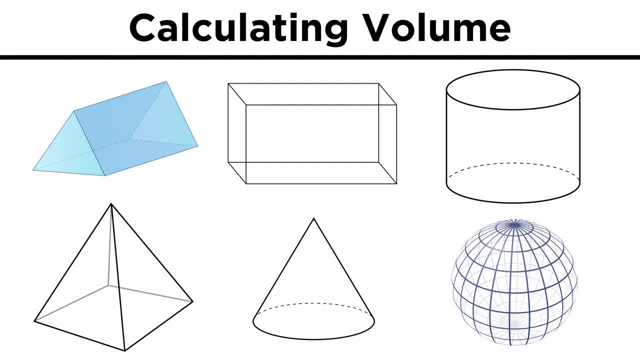 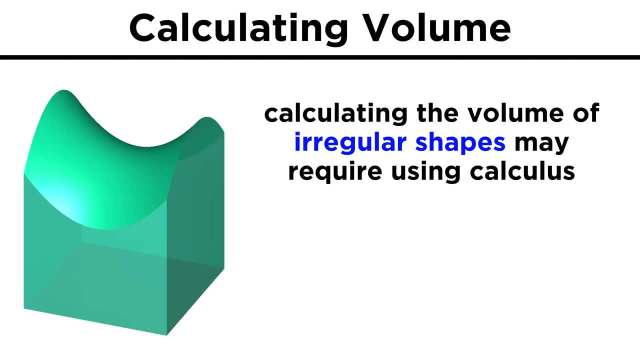 and multiply by four to get thirty six times pi is thirty six pi cubic meters. These are most of the regular shapes for which we have reliable equations to calculate volume. There are, of course, many irregular shapes that have a more unpredictable curvature.